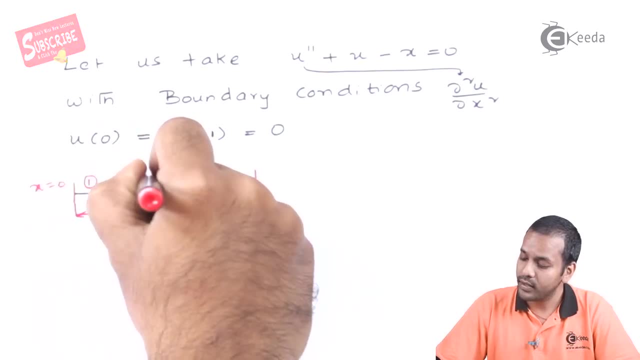 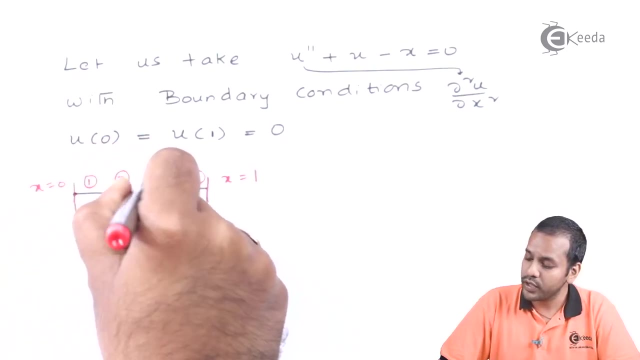 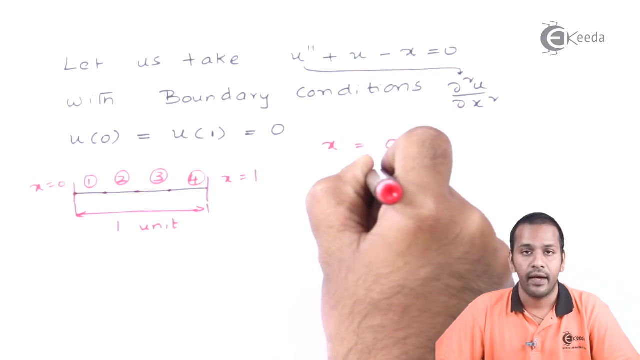 Let us say this is my first unit, second, third and fourth. So we are having 5 grid points here: 1, 2, 3, 4, 5.. Okay, so where the first grid point lies at x, equal to 0, and the second grid point at 0.25, 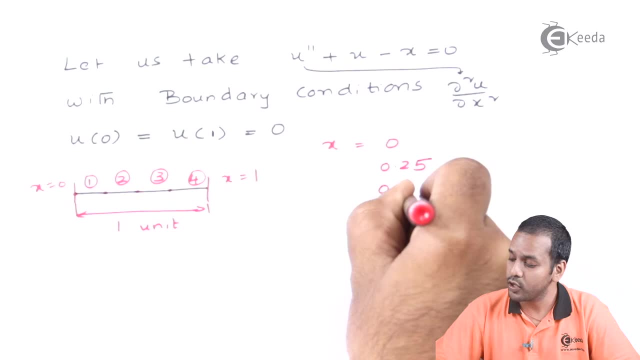 and third grid point at 0.5, and fourth grid point at 0.75 and fifth grid point is at 1.. So these are the positions of the grid points. Okay, so now how to solve this differential equation using finite difference method is: 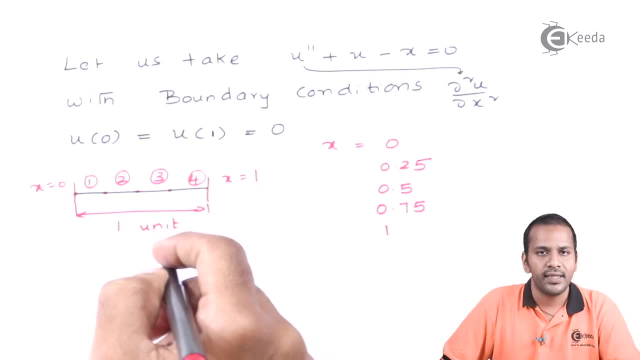 we will approximate our differentiation using the Taylor series and we will replace them in our differential equation. So these approximations are of different kinds. So we are having forward approximation, forward difference, backward difference, central difference. So depending on the accuracy we want, we can use those approximations. 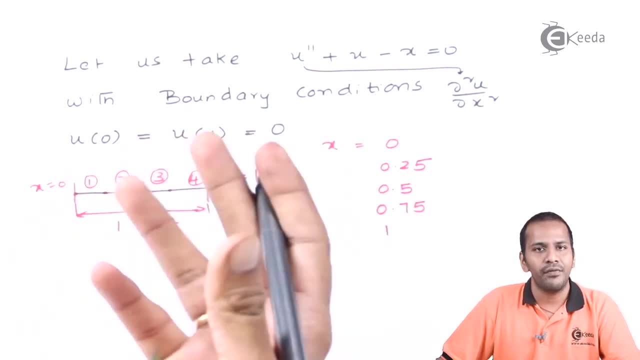 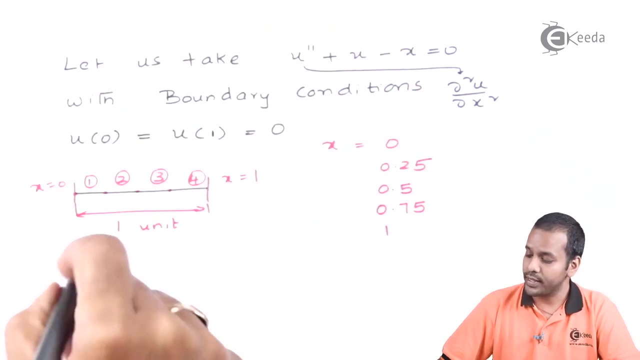 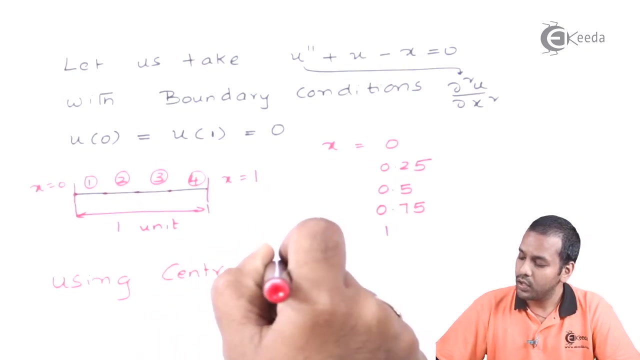 we can substitute them in our differential equation and we can convert this differential equation into an algebraic form. Okay, so right now, let us use central difference technique and replace this second order term into an algebraic term. So let us use using central difference. 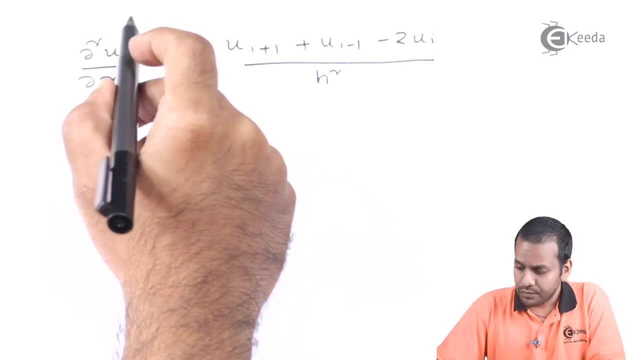 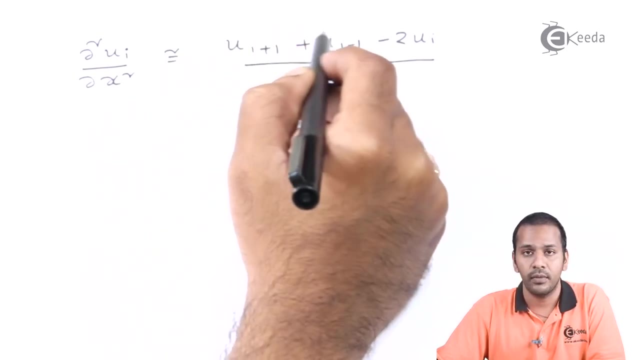 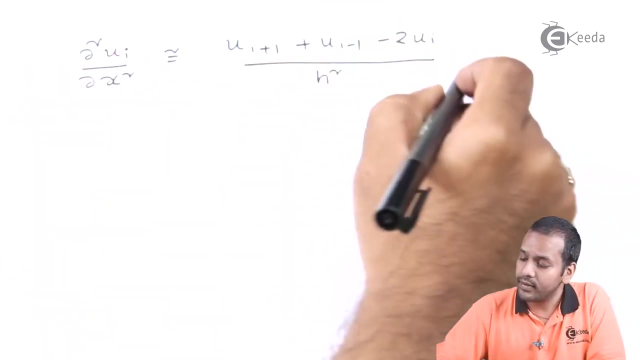 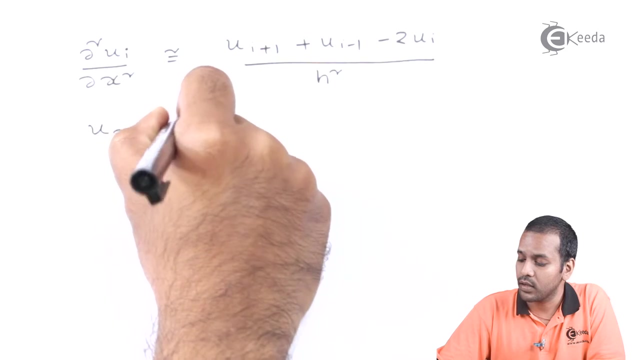 So, according to central difference method, we can approximate this second order term, that dou square ui by dou x square as ui plus 1 plus ui minus 1 minus 2 ui by h square Right. So let us apply this one in our ordinary differential equation, that is uxx plus u minus x. 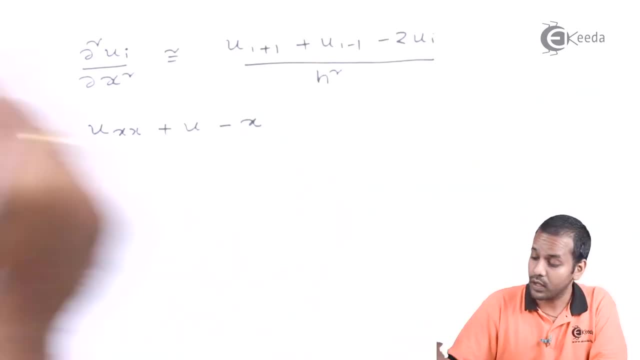 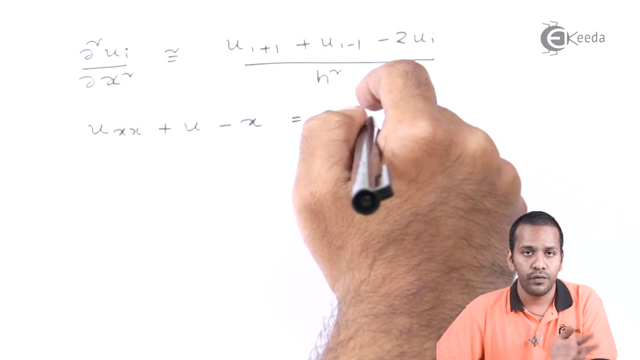 So what I wrote? is it plus x or minus x? It is minus x here. Minus x is equal to 0.. So we have to apply this equation at each and every node of the interior nodes, because at the exterior nodes we know the values. 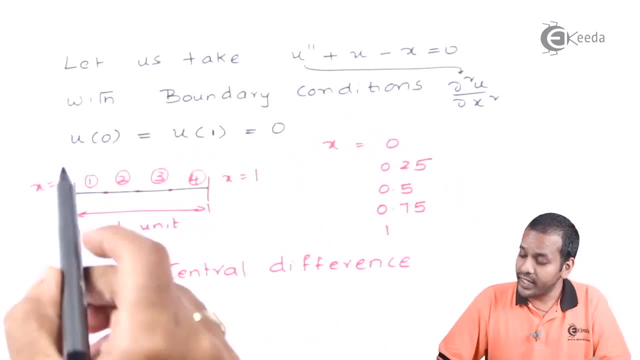 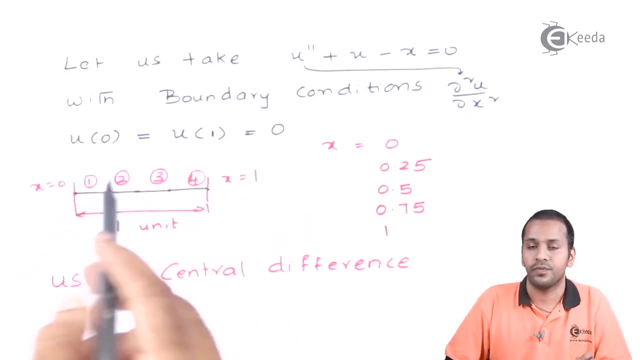 Right. The boundary conditions are already given At the exterior nodes, at the exterior grid points. that is, at x is equal to 0 and at x is equal to 1. we are already having the values as 0. So we want to know the values at the interior points. 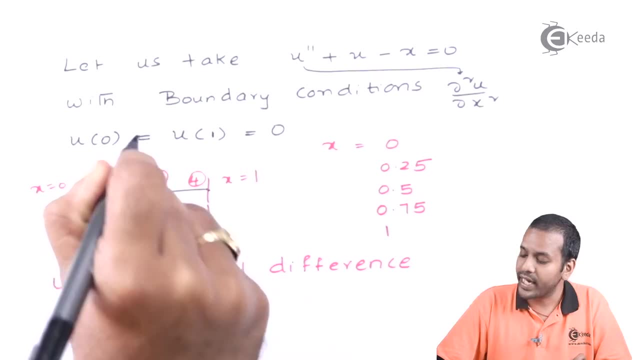 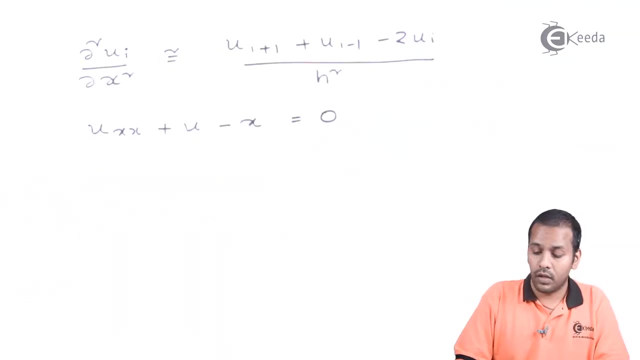 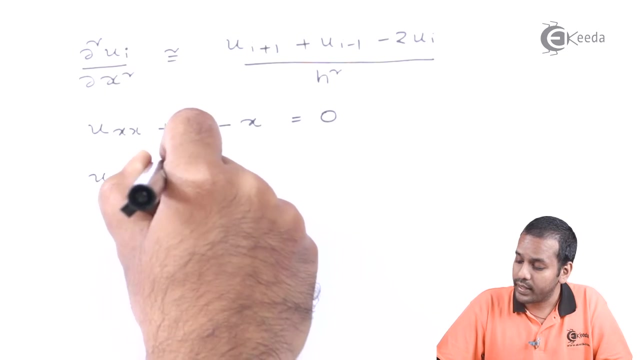 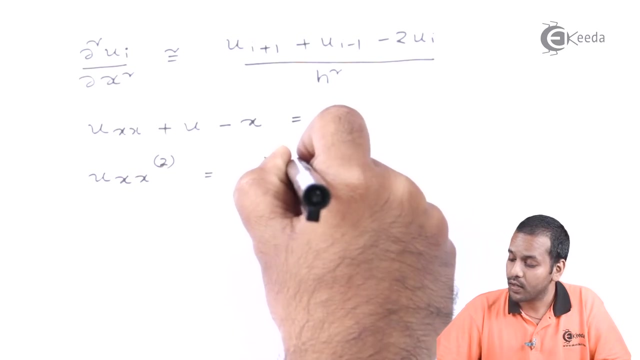 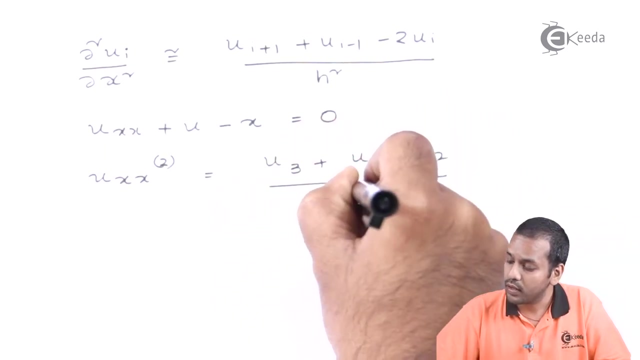 Right, So I want the value at second grid node and third grid node and fourth grid node. Okay, Fine, So at the second grid node, at the second grid node can be approximated as u3 plus u1 minus 2u2 by h square. 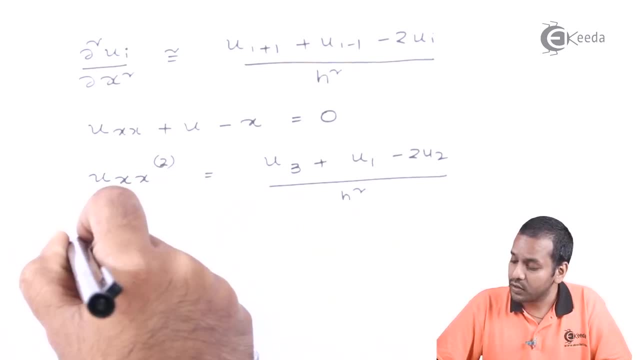 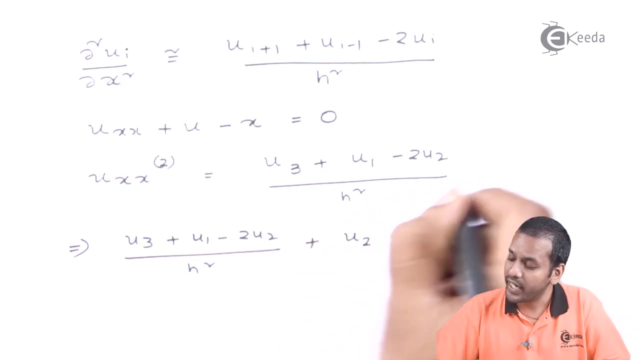 Right. So substituting this in the governing equation that implies u3 plus u1 minus 2u2 by h square plus, this is at the second grid node, u2 minus. the second grid node is located at the position h, equal to 0.. 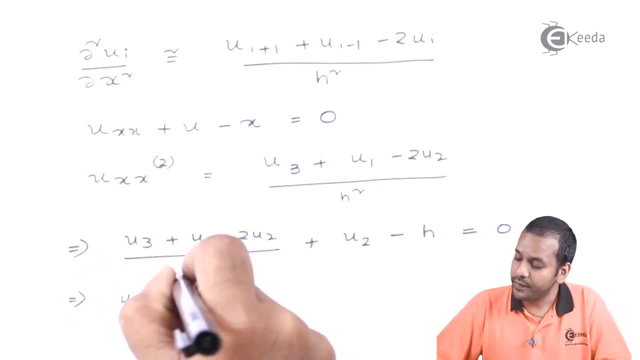 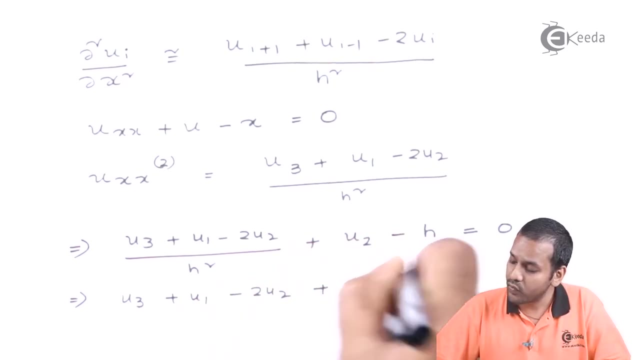 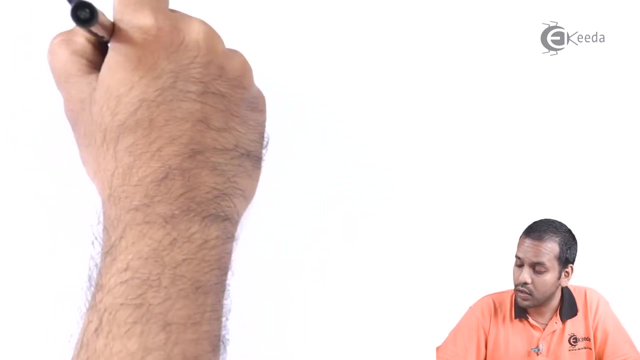 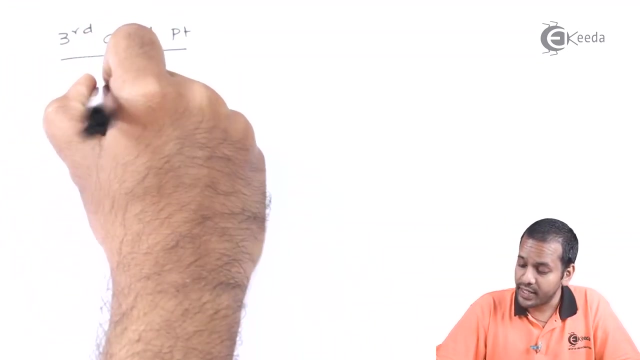 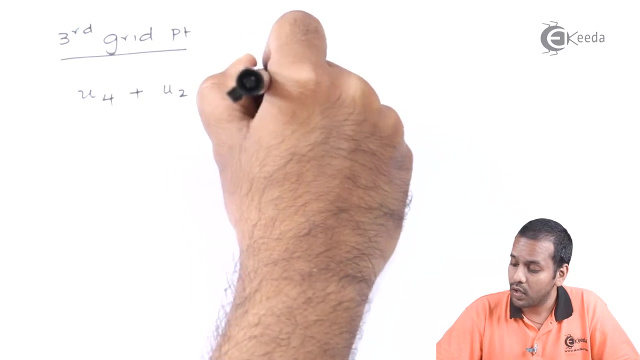 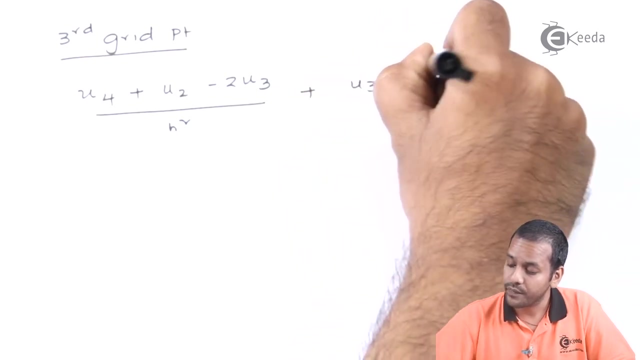 So this equation will become u3 plus u1 minus 2u2 plus h square u2 minus h cube is equal to 0. So let us say this is our first equation. If you apply for the third grid point, what we will write is u4 plus u2 minus 2u3 by h square plus u3 minus h. 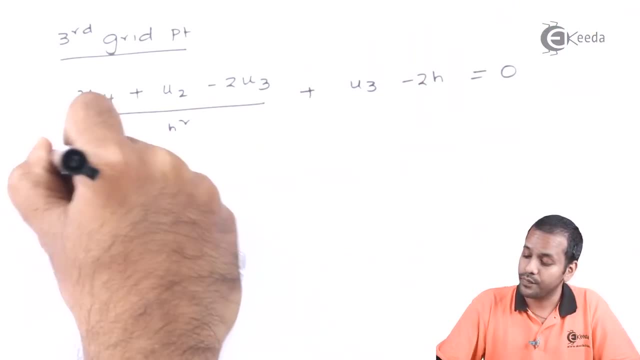 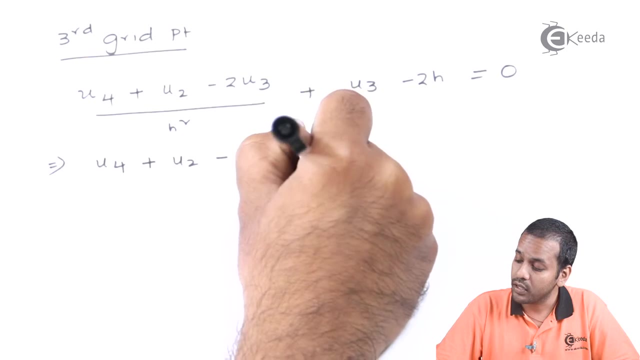 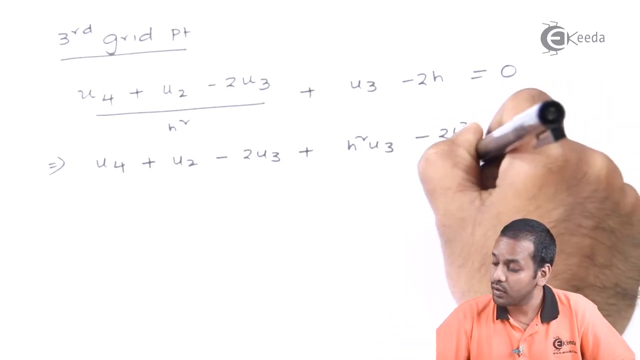 Is it h or 2h? It is 2h equal to 0.. So this is nothing but u4 plus u2 minus 2u3 plus h. square u3 minus 2h cube is equal to 0.. Let us call this as second equation. 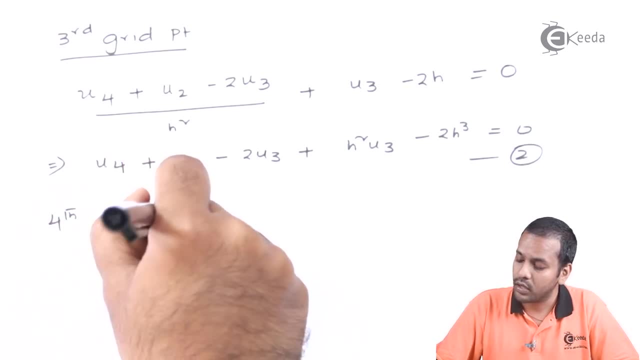 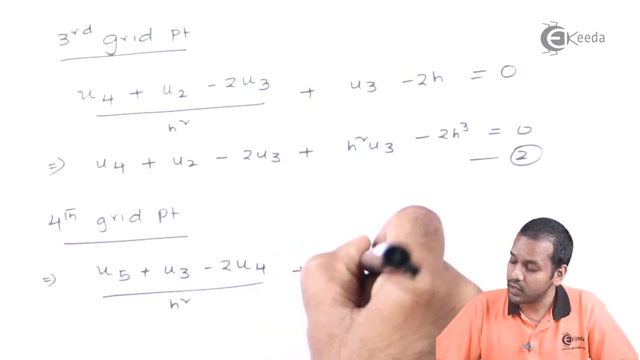 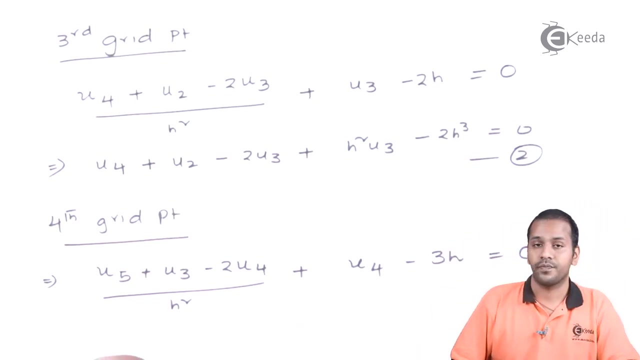 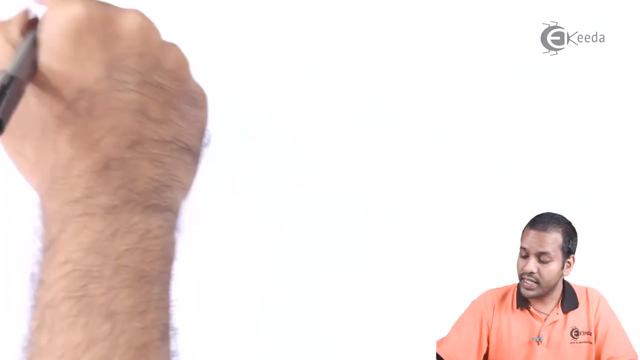 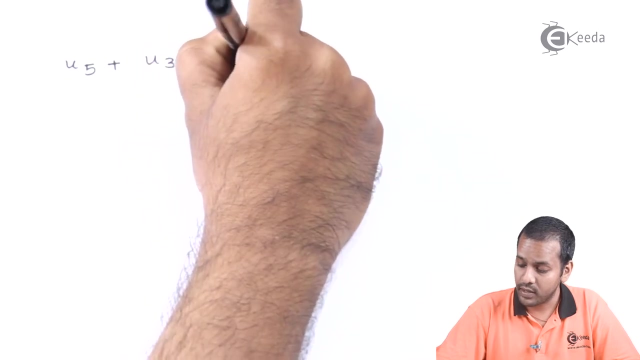 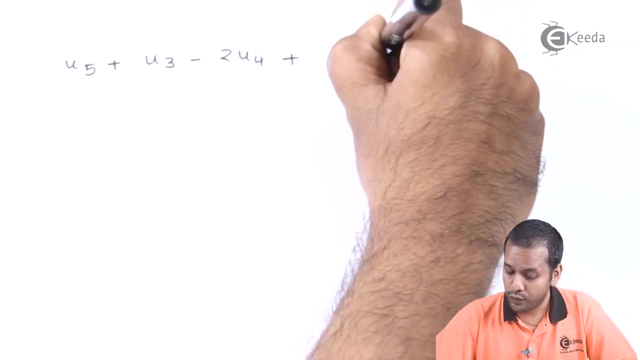 Similarly at the fourth grid point it is u5 plus u3 minus 2u4. by h square plus u4 minus 3h is equal to 0.. Right, So this can be written as u5 plus u3 minus 2u4 plus u4h square minus 3h cube is equal to 0.. 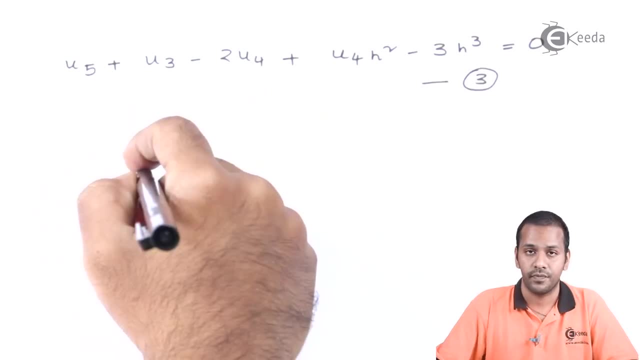 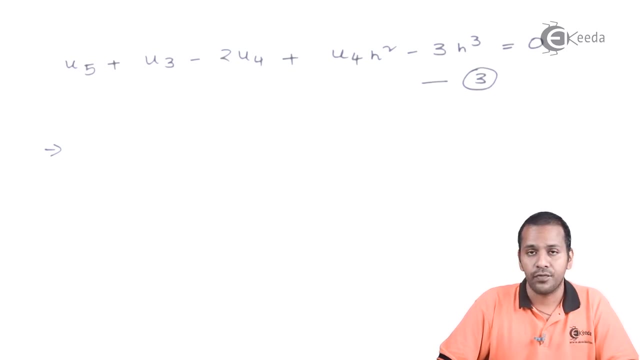 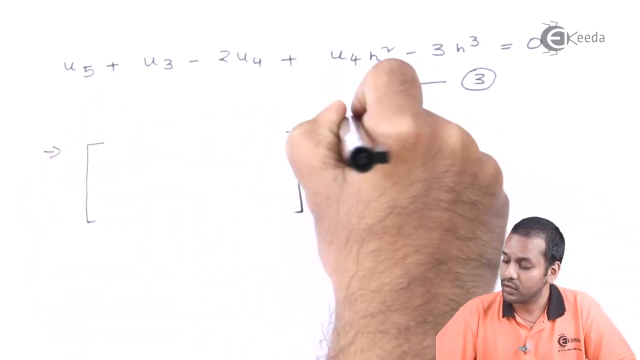 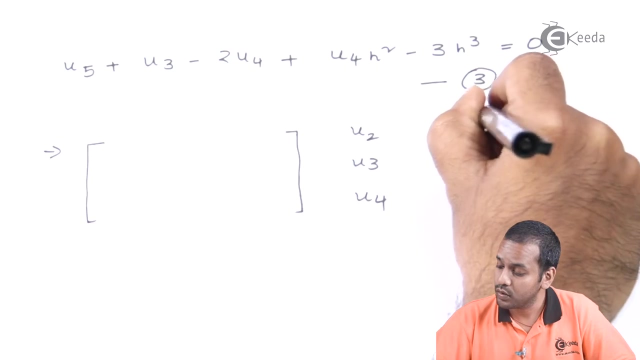 So let us say this is my third expression. So if you combine all expressions then you can put it in the matrix form For sure. So you can write in this fashion: u2, u3, u4 is equal to some other vector form. 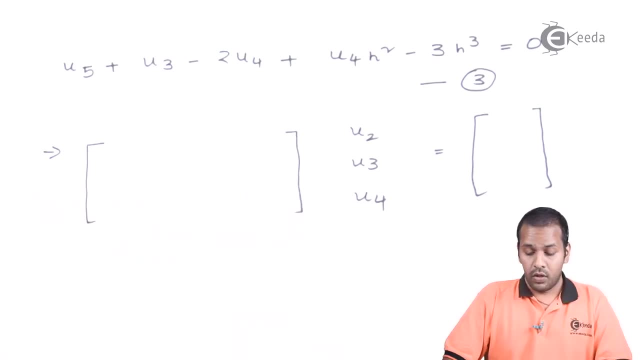 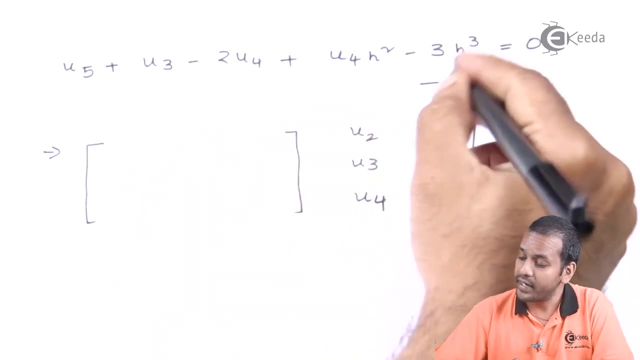 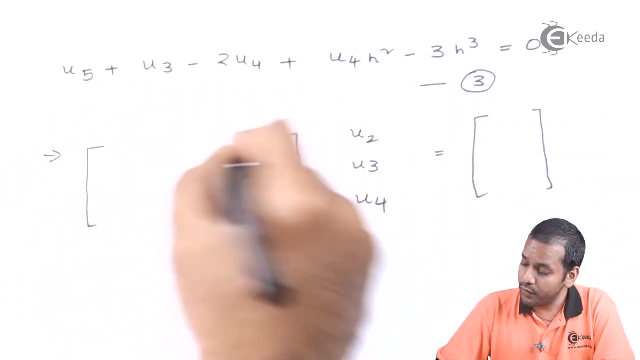 So can we fill this in the matrix form? Yes, So from the first equation, what we can write is: so just fill up these matrices and we can calculate u2, u3, u4 using some algebraic technique. Okay, So shall we fill these things? 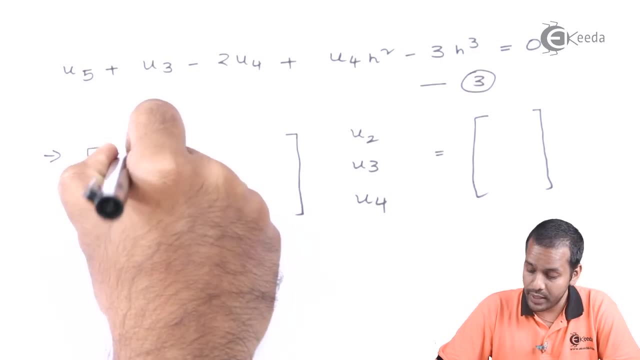 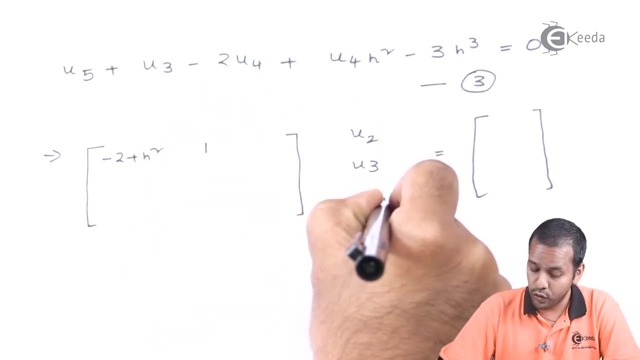 So what is the coefficient of u2 from the first equation? It is minus 2 plus h square. And what is the coefficient of u3? It is 1.. And what is the coefficient of u4? It is 0.. And what will come on the right hand side? 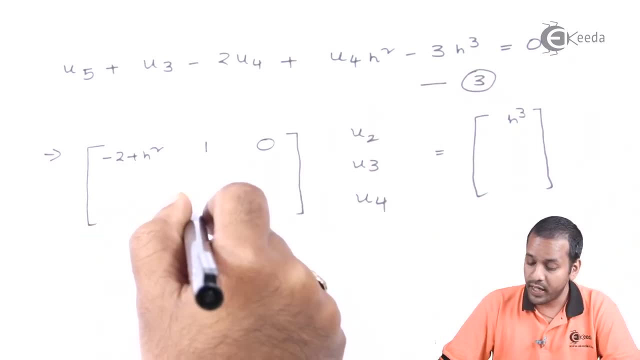 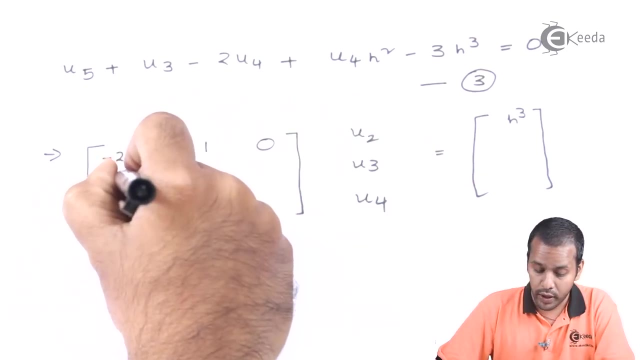 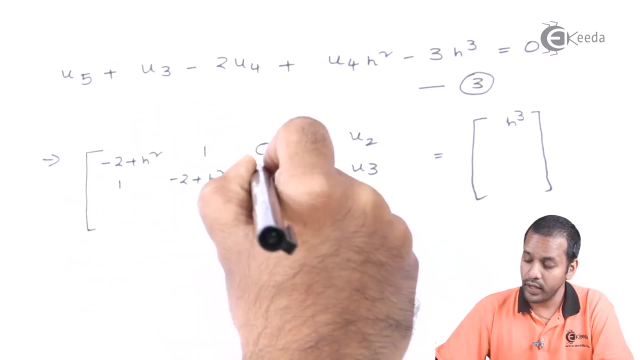 It is h cube. Similarly, if you fill the coefficients from the second expression, what is the coefficient of u2? It is 1.. Coefficient of u3 minus 2 plus h square And coefficient of u4 is 1.. And on the right hand side, 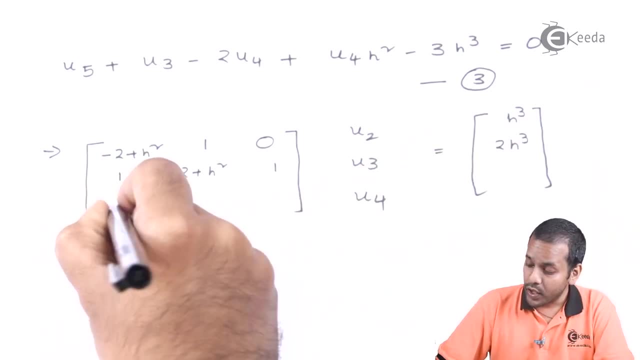 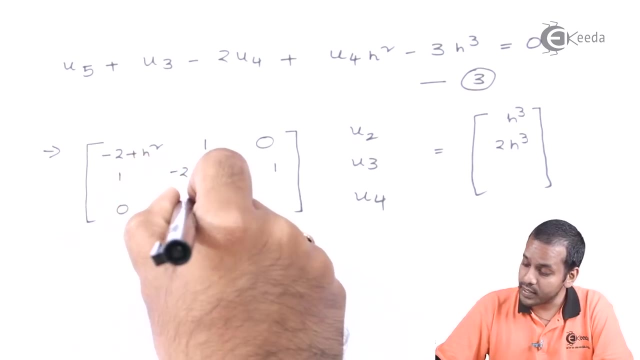 you are having 2 h cube. Similarly for the third equation: what is the coefficient of u2? 0.. Coefficient of u3 is 1. And coefficient of u4 is minus 2, plus h square. And on the right hand side. 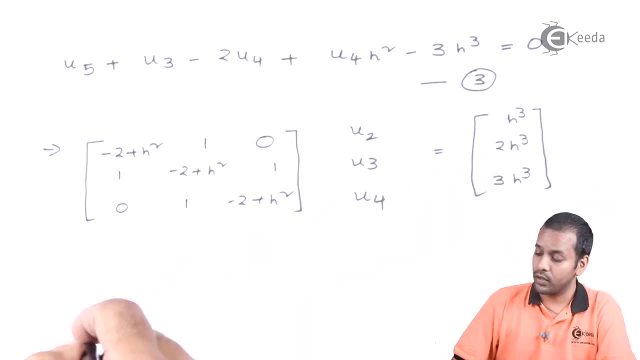 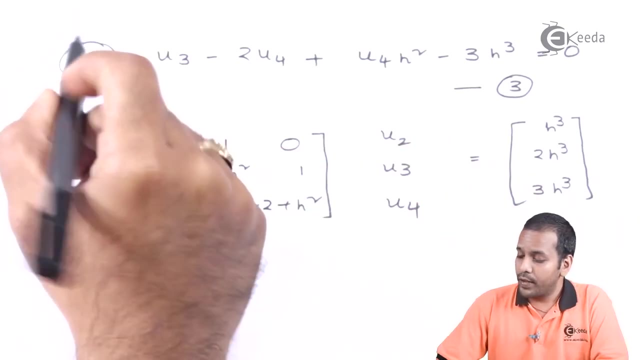 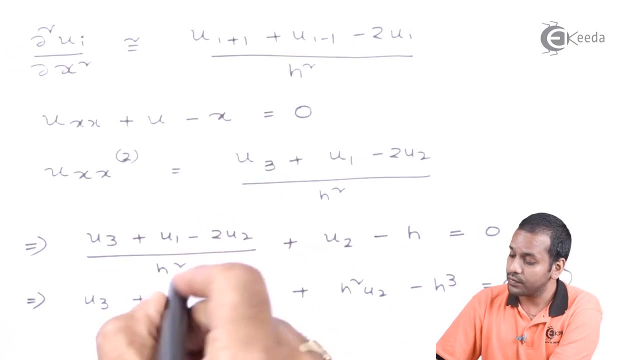 we will be having 3 h cube. Okay So, but what happened to this u5?? So, this is the matrix form of the above three equations, But what happened to this u5, as well as u1 in the first expression? What about this u1?? 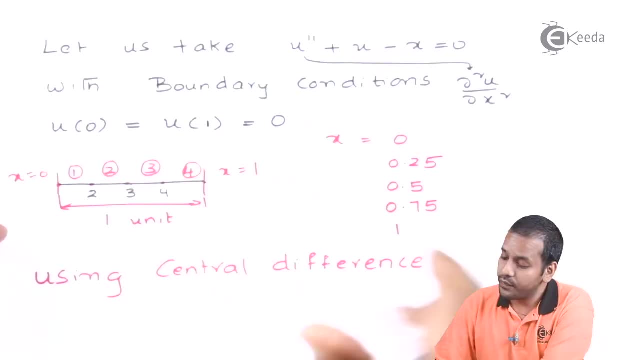 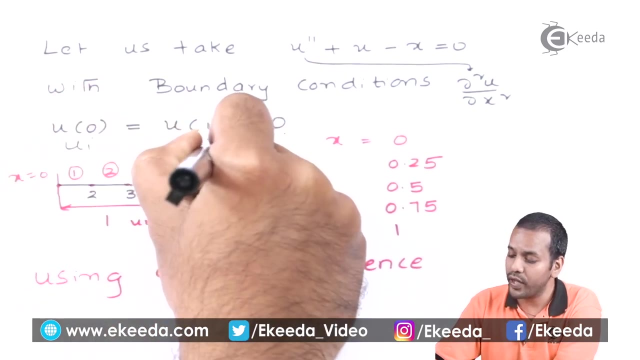 We know already these values. Right, These are the boundary conditions. These are the boundary conditions already given: u at 0 and u at 1, equal to 0. That is, u1 and u5 are already given. So there, anyway, they are 0.. 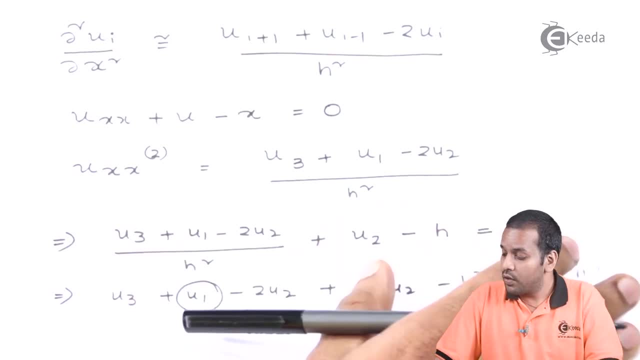 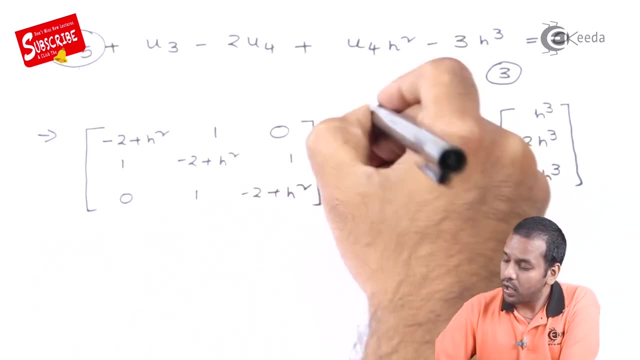 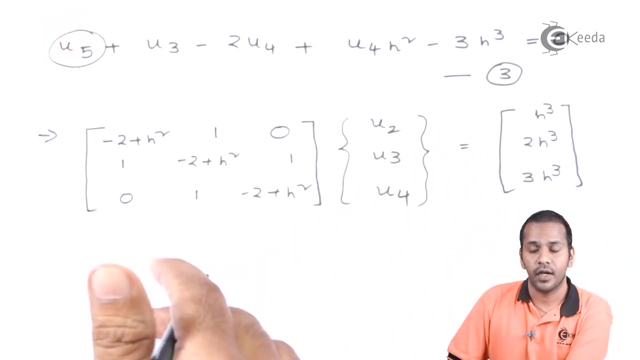 So they won't hurt our solution. Fine, That is, we have used the boundary conditions here. If you observe- And these are the unknowns- we need to calculate u2, u3, u4. Just invert this matrix. Keep this h value. 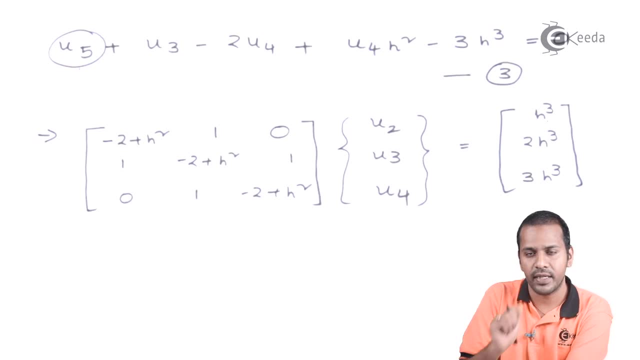 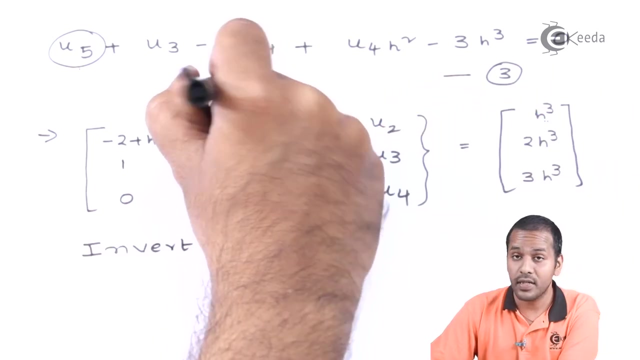 h value is nothing but that element size, Each element size. If you assume each element size is uniform, then it is an uniform mesh or uniform grid. So just substitute this h value and invert this matrix, Then you will get u2, u3, u4.. 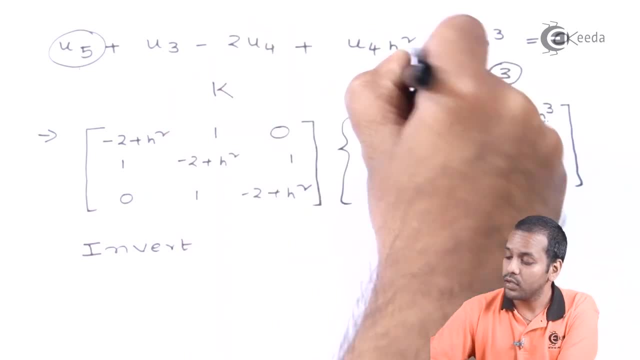 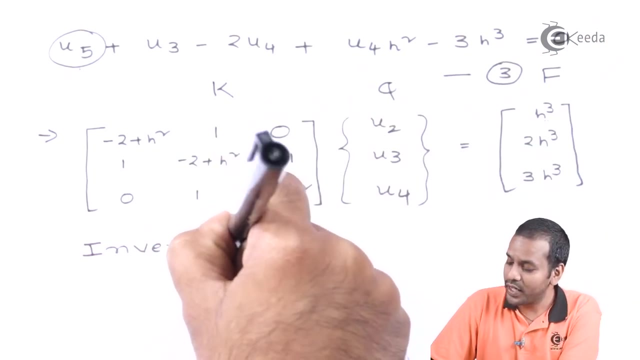 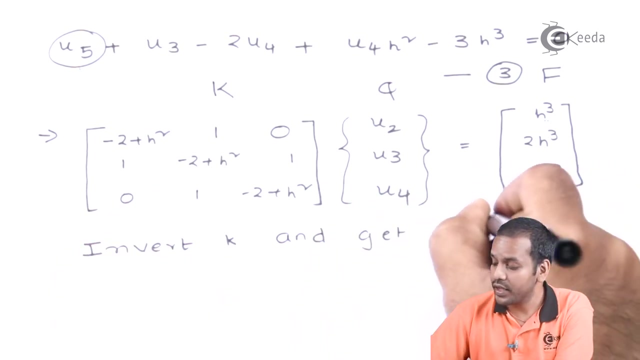 So what is this form? If you remember starting of this lecture, Isn't it? This is in the form of: kq is equal to f, Right, So invert k and get q, Which are the unknowns. Okay, Fine, So. 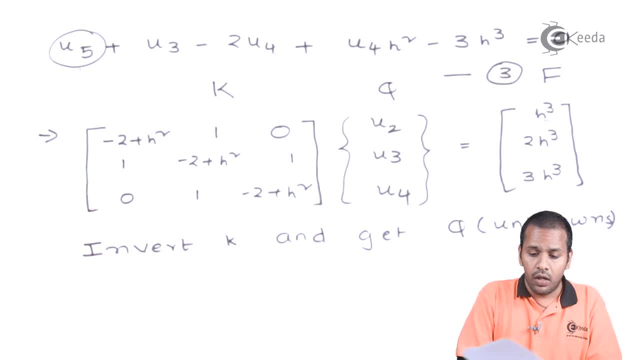 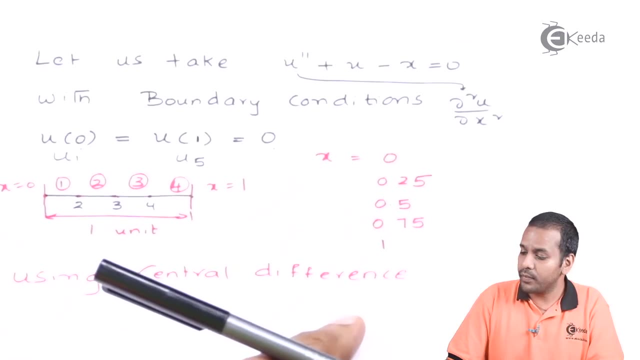 this is finite difference method. But what is the drawback of this finite difference method? Why we want to go to finite element method? Already we are having a numerical method, which is very well established finite difference method, But why we want to go to finite element method? 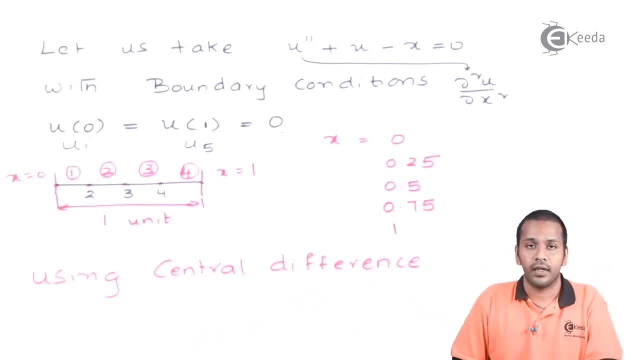 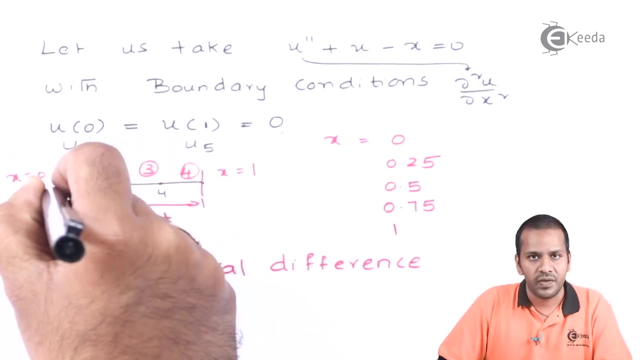 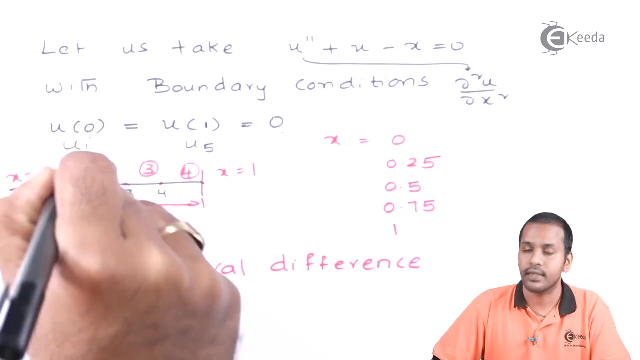 The very reason we can say is: what if we are having gradient boundary conditions? What if I am having, instead of x is equal to 0 here? what if I have some dou u by dou x or dou square u by dou x square? If you want to give the boundary conditions,